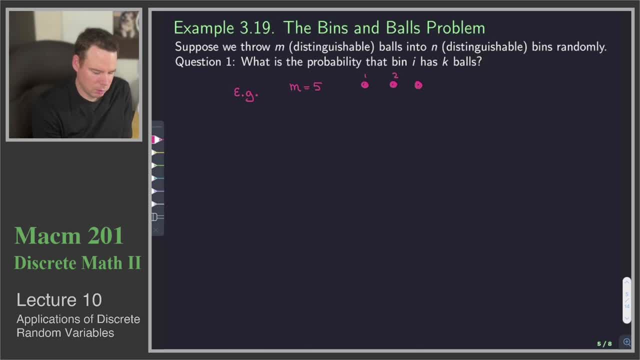 one, two, three, four, five. and let's say we've got n equals four, so we've got four bins to put them in. so bin one, bin two, bin three and bin four. And since they're distinguishable, it means we can imagine they're all labeled or they all have. 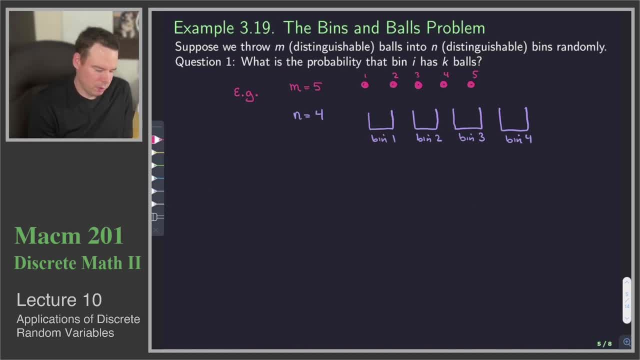 numbers And we're interested in the ways of distributing these balls into these bins. In particular, we want to know, you know, if we do a random distribution, what's the probability that one of these bins, bin i, has exactly k balls in it. So an example of a distribution could be. 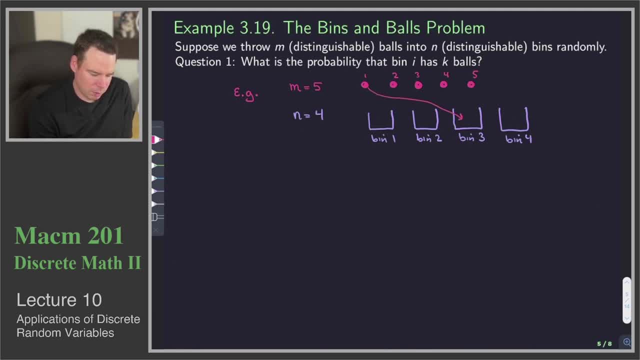 ball one could end up in bin three, ball two could also end up in bin three. So there was a, a sample, and so maybe I'll just put the numbers of what was in here. So we had four was in there, and then we had three. 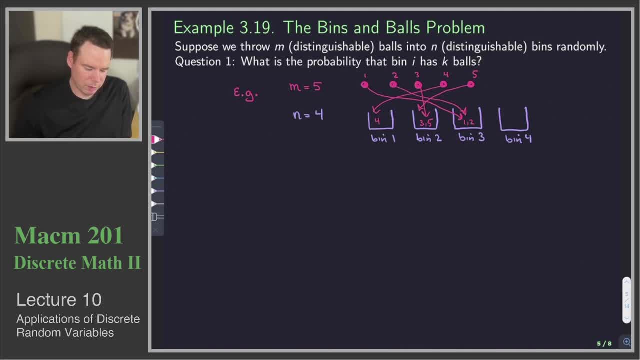 So d and b and d and 3 and 5 landed in here And one and two landed in here. It just turned out that there was a bin that was empty and one bin had one. two bins each had two balls in them. So that's the idea of distributing the balls into the bins, and we want to know. 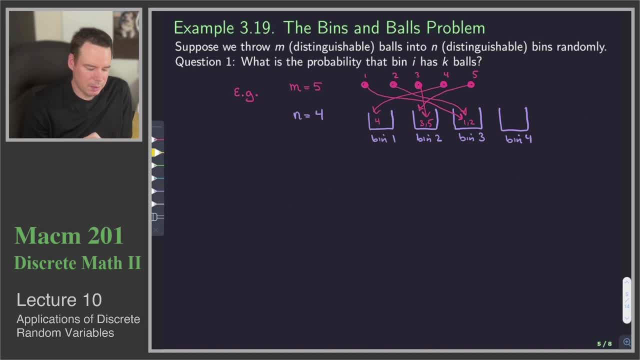 some answers to some problems about this. So the first one is: what is the probability that bin i has k balls? So We're imagining i has k balls, this is fixed. So this is some bin we've just fixed. It could be bin 3, for example. 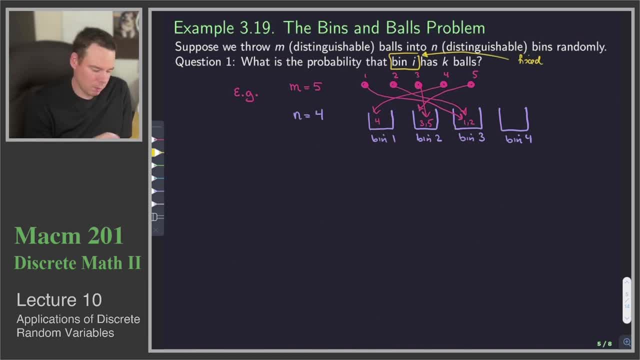 What's the probability that bin 3 has k balls? So that's how we're going to start this off. We're going to fix i somewhere between 1 and n. Now we're interested in the number of balls that bin i has. So we could, for example, let y i be the 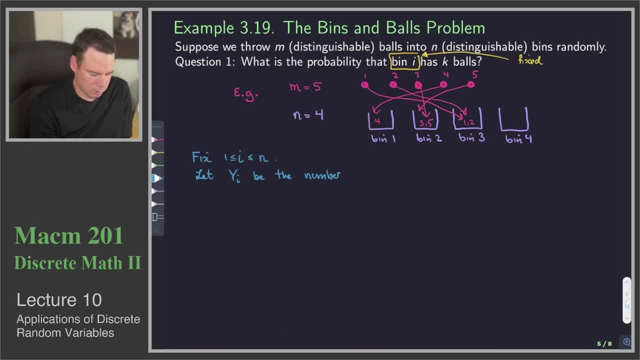 number of balls in bin i. And so what are we interested in? Well, we want to know what is the probability that we can get the number of balls with in a number of a balls has. Ok, Let's check. let me do that again. 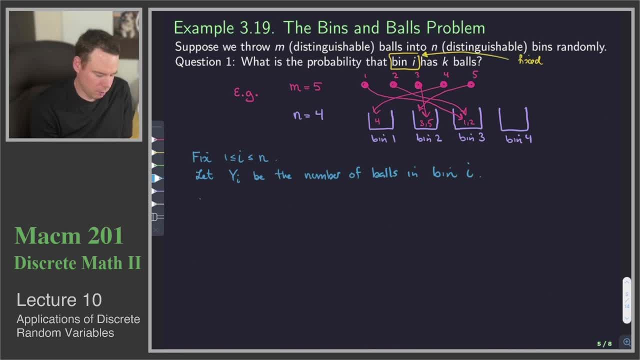 that yi is equal to k. So let's get a feel for what these probabilities are. What's the probability that yi is equal to zero? What's the probability that, when you distribute these balls into the bins, that this particular bin i gets zero balls? Well, what this means is that the m balls ended up being distributed over n. 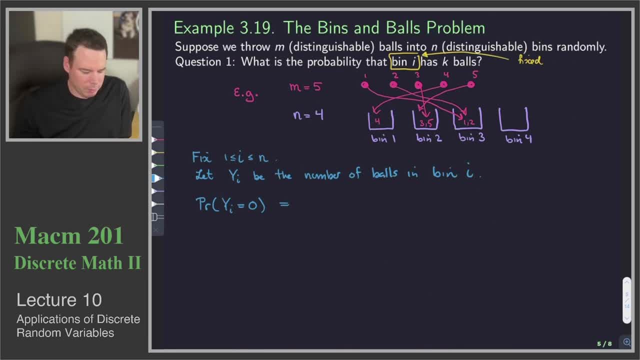 minus one containers. So I look back at this diagram and I think: is there a way to extract from this diagram a way to represent it as an object that I know how to count? And the idea is, absolutely I can, I can think of it as you know one. 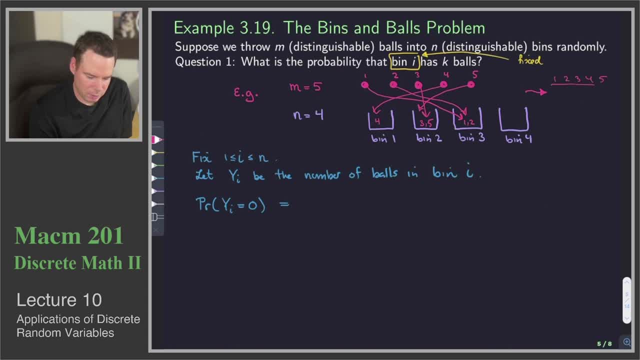 two, three, four, five as the balls, and then underneath that I just write the bin they went. So this would have been three, three, and then ball three went to bin two, ball four went to bin one and five went to bin two. So I can encode it as this string: three. 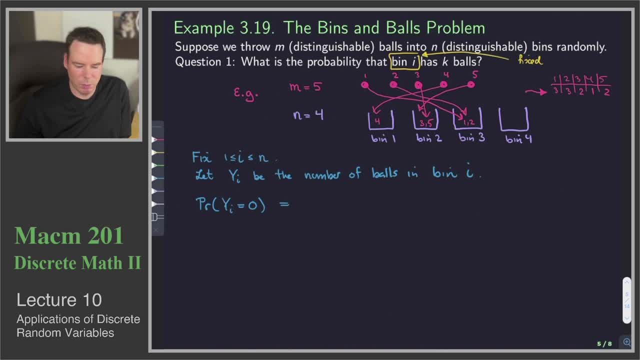 three, two, one, two. That tells me exactly where balls one through five went, and I can use that to help me figure out what the probability of yi being zero is. What's the probability that the ith bin has no balls in it? Well, it means the m balls had to get distributed amongst the n minus one. 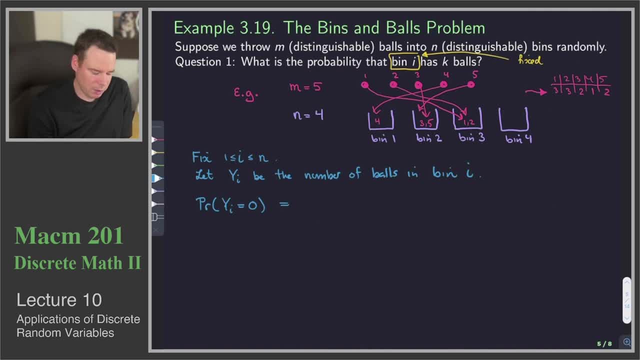 bins. So that means: for ball one, there are n minus one choices for it. For ball two, there are n minus one choices for it. All the way up to ball m, there are n minus one choices for it, because I'm avoiding putting it in bin i. 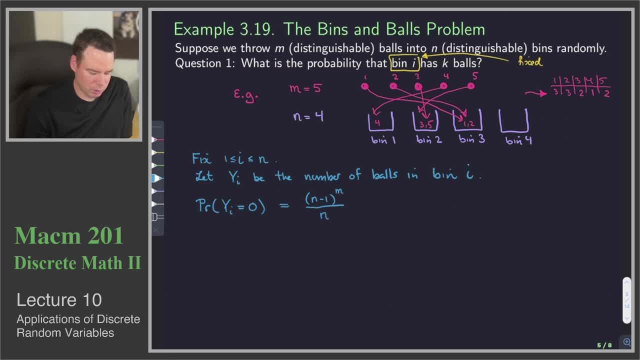 And that's going to be divided by the total number of arrangements I get, and that is there are n choices for every ball, So that would be n to the m. So this is- I'll put it in a different color- this is ways to distribute balls and 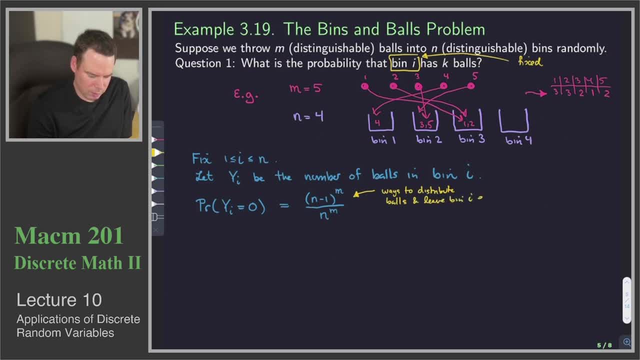 leave balls bin i empty, and this is the size of sample space, The unrestricted ways to distribute the balls across the n bins. So there we go. We've got our value and we could simplify it a little bit perhaps. Maybe I could write it as a one minus one. 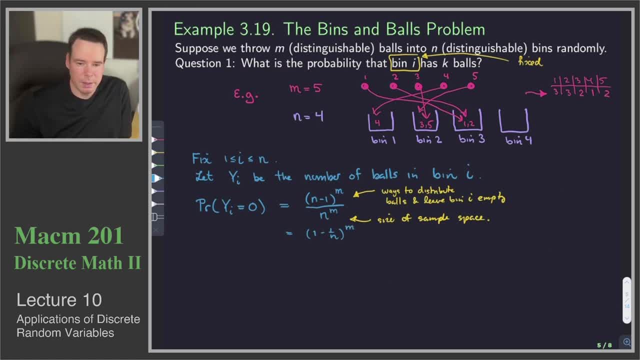 over n to the m. Now how about the next one: Probability that y- i is equal to one. Ultimately, we're interested in what is the probability that bin i has k balls. So we want to know what is the probability that y i is k. We're going. 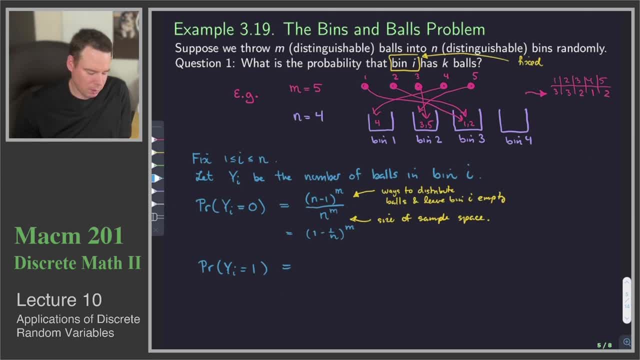 to work our way up there. So this says that the bin i has to have one ball in it. Ok, so how do we figure this out? Well, how many different arrangements are there? that has bin i with one ball. Well, what I could do is I could think of how many ways could I distribute the 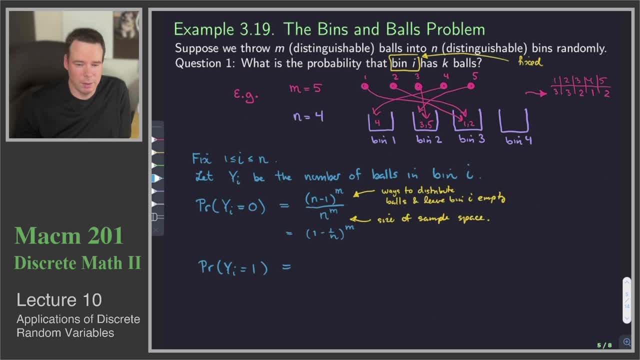 balls, so that bin i has one in it. Well, first I could pick the ball that I want to go in it. So there are m choices for the ball that I want to go in bin i, and then the remaining m minus one balls can get put in any of the n minus one containers. So there are n minus one. 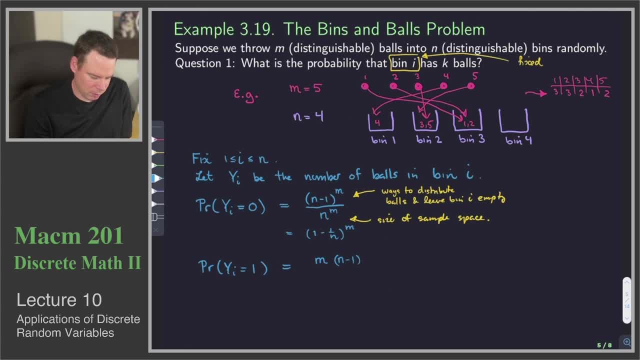 choices for the next ball And the next one, and the next one. so I got n minus one to the m minus one And that's all over the number of ways, or the size of the sample space. I guess I more succinctly put it. i was going to say the number of ways to spread out the 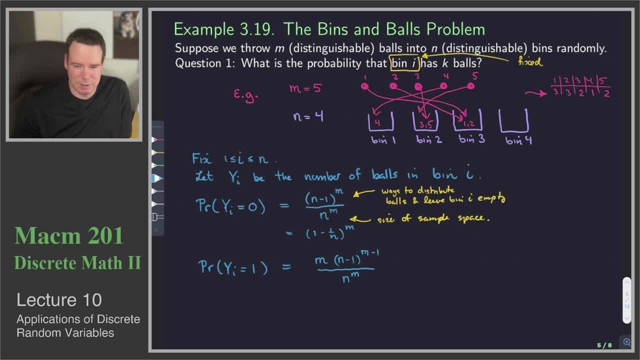 balls without any conditions. But that's just the size of the sample space. So there we go. We can think of it. you know, a little bit more generally, as I chose a ball to put in bin i and then I've got this 1 over n- I'm just rewriting this in a slightly different way- and then the m minus 1. 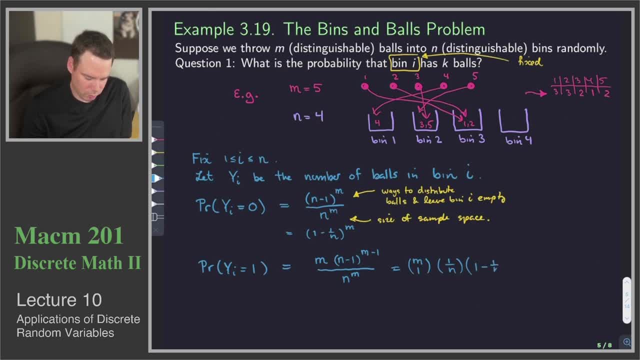 I could write as the 1 minus 1 over n to the m minus 1.. So I could rewrite that expression in this way. and the way this is really telling me that to think about the probability is that: what's the probability? that bin i has one ball. It's the number of ways it could have one ball. 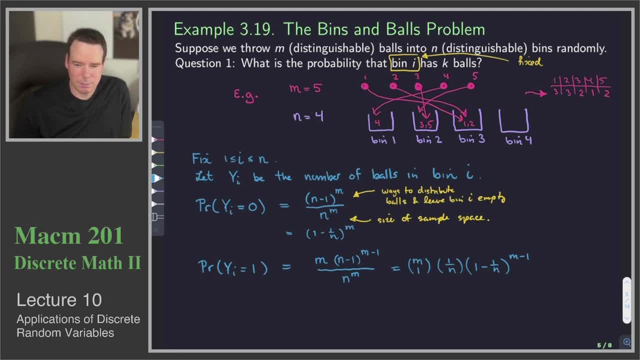 that is, of any of the m balls, you can pick one of them to put in there. the probability that that particular ball that you've chosen, that you want to get into bin i, the probability that it actually gets into bin i- is the 1 over n, and then the 1 minus 1 over n to the m minus 1 is the. 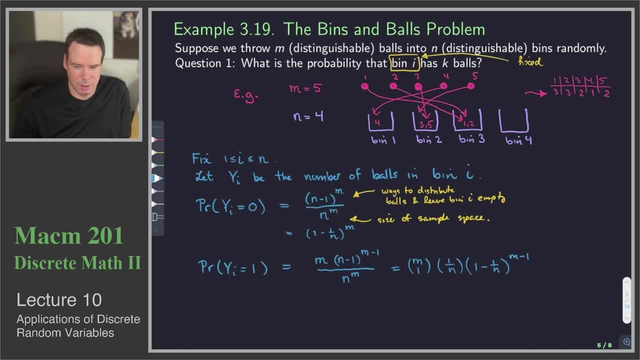 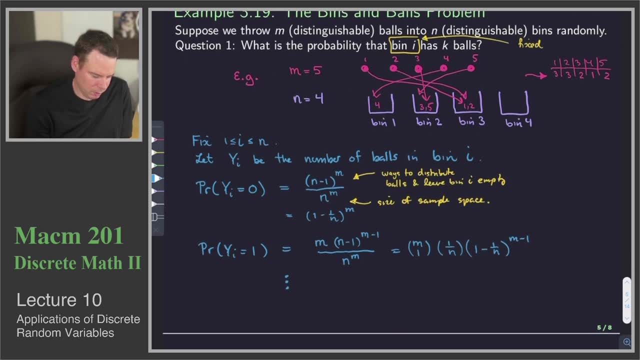 probability that it actually gets into bin i. So I could write this as the 1 minus 1 over n to the, but all the remaining balls miss bin i. So that's another way to think about it, And so what this tells me, then, is that, in general, 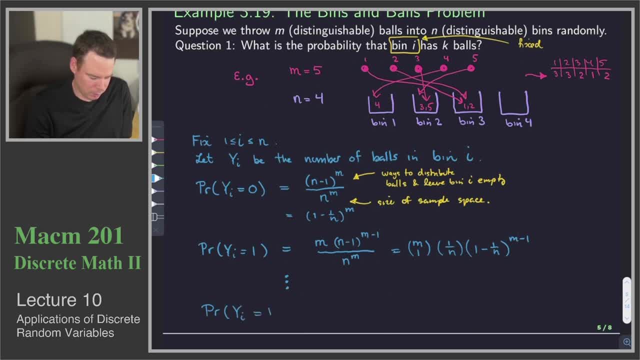 what's the probability that bin i will contain k balls? Well, I'll think about it in terms of the number of outcomes that has bin i containing k balls- and that is the number of ways it could have k balls- is choose the k balls to go into bin i. Once you've chosen those balls, then the remaining balls, which? 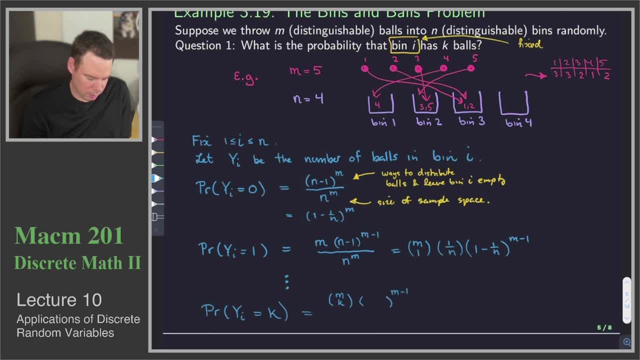 are m minus k of them. they can go into any of the remaining n minus 1 bins. So you've got n minus 1 choices for the n minus 1 bins. So you've got n minus 1 choices for the m minus 1 bins. 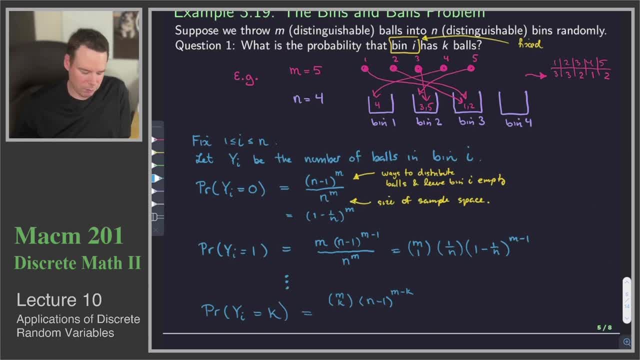 next ball, n minus 1 for the next one, and so on, all the way down for those balls that aren't going to end up in bin i and all that's over. n to the m, or again we could rewrite it as m choose k, 1 over n. 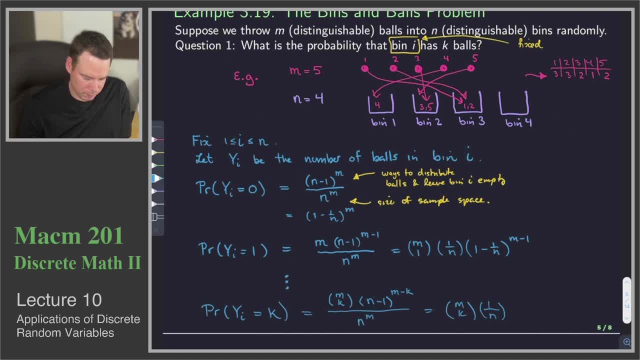 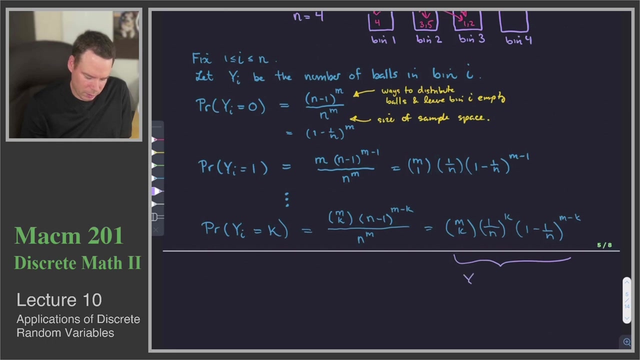 to the k, 1 minus 1 over n to the m minus k. so that's another way we could write that expression. and when we write it in this way, what do we see? we see that y- i is binomially distributed. so the probability distribution for this random variable, y- i, 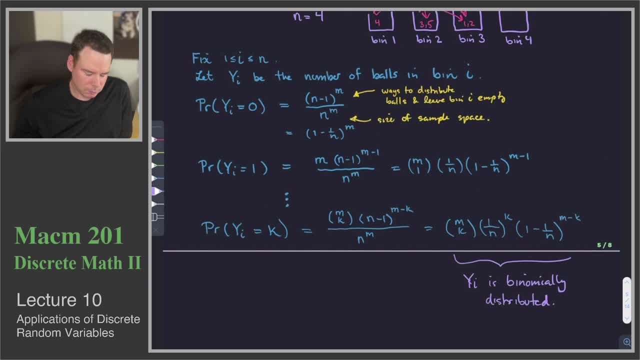 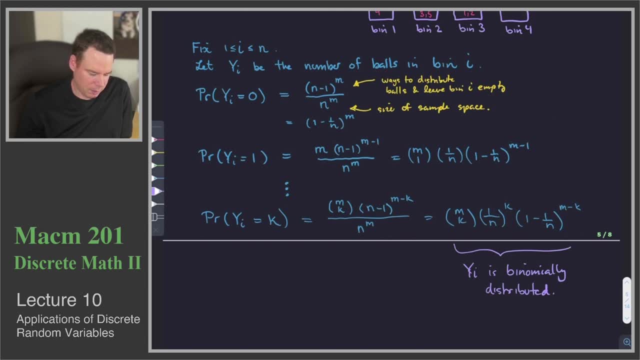 actually turns out to be a binomial distribution, as we can see there. all right, so we've worked out the probability that bin i has exactly k balls and that's it right there. or instructions you can think about in this way as well. either of these are equivalent to think about. okay, what is? 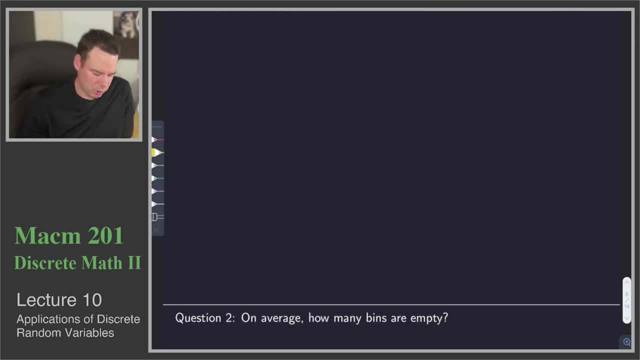 the next question. the next question is asking us, on average, how many bins are empty. so we distribute the balls, we get a number of empty bins perhaps. so, on average, how many empty bins do we expect to get? let's just draw out an example to see what we're dealing with here. 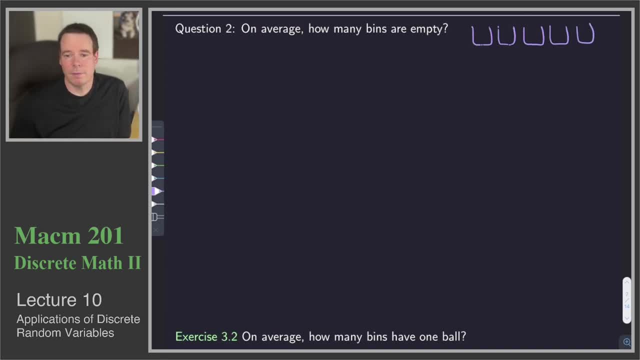 so let's just say we've got five bins in this case and we've distributed some balls amongst those bins. so i got a ball here, maybe i have three of them there, and then i've got another one over here. the balls would be numbered, the bins are numbered. 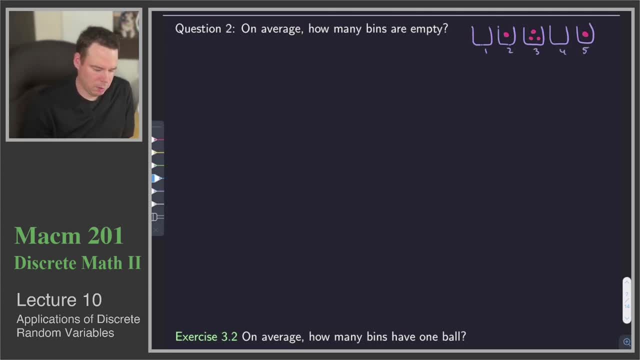 and i'm interested in how many bins are empty. so let's just draw out an example to see what we're dealing with here. so that means i'm really interested in a random variable that takes some distribution of balls into bins and returns the number of empty bins. so in this case it would return two. 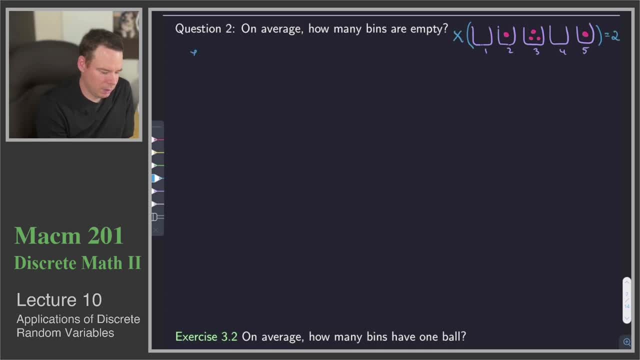 so that's the random variable i'm interested in. so let x be the number of empty bins. so, in order to deal with this, what i'm going to do is i'm going to introduce a few more random variables. so let x, i, where i goes from one to n, and what it's going to do it's going to be kind of like the random. 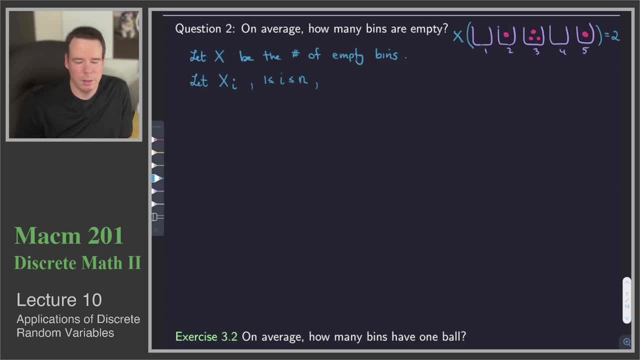 variable we introduced above y i, where y i returned the number of balls in a bin. in this case, i don't really care about the number of balls in the bin, i'm just going to do a little bit more, and then i'm just interested in empty, not empty. so in this case, x i is going to be the random. 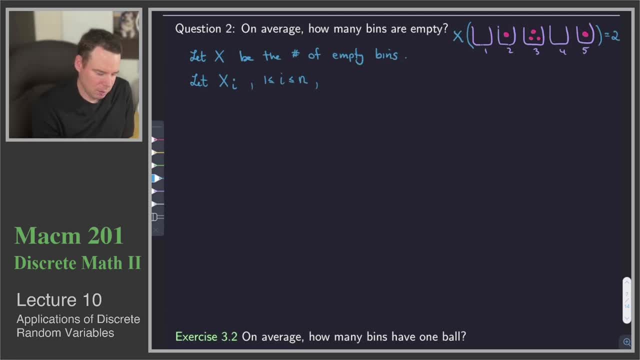 variable which just indicates whether the bin is empty or not. so let x i be the random variable given as follows. so x i of our element in our sample space. so some arrangement of balls to bins, returns, returns, returns, returns, returns 1 if bin i is empty and 0 if bin i is not empty. 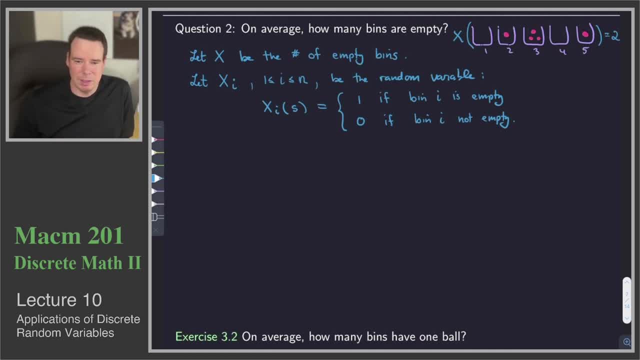 So notice here: 1 indicates empty, 0 not empty, because we're interested in empty bins. So that's my valuable piece of information. What are the empty ones? That's why I've assigned a 1 as an indicator there. 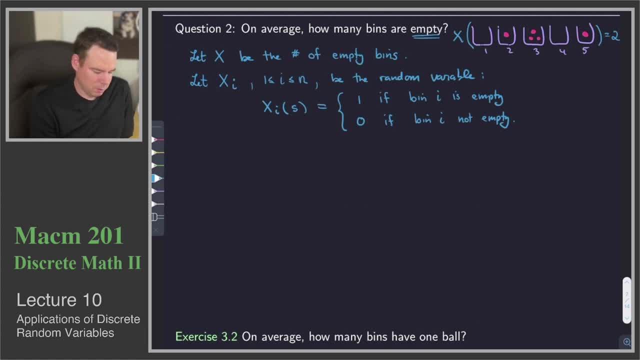 1 if it's empty. And so then what I notice is that, well, maybe we can do a brief example of this. We'll take our 5-bin example from above and we'll throw the balls in there, Something like this: 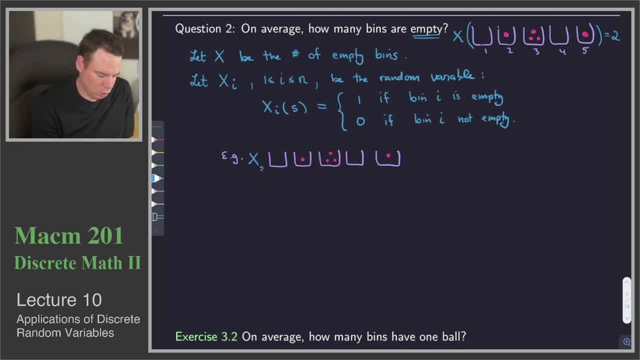 Then I could ask you know what is x2 of this? Well, x2 is asking for the indicator of: is the bin empty or not? So you can think of it as a Boolean Empty or not. So I scan across and say that's a 2.. 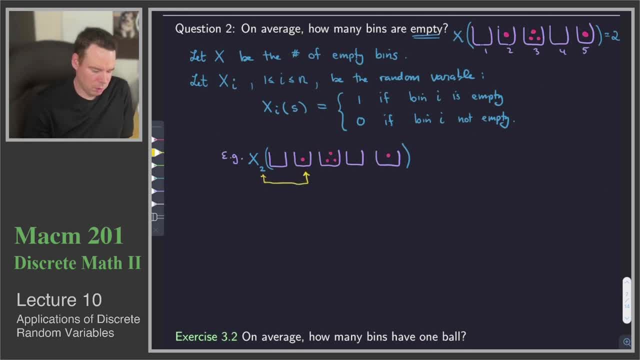 So it's really asking about bin 2.. Bin 2, not empty. Therefore, the value comes back as 0.. As opposed to, maybe, if I ask about bin 1.. In this case, we'll redraw our arrangement of balls. 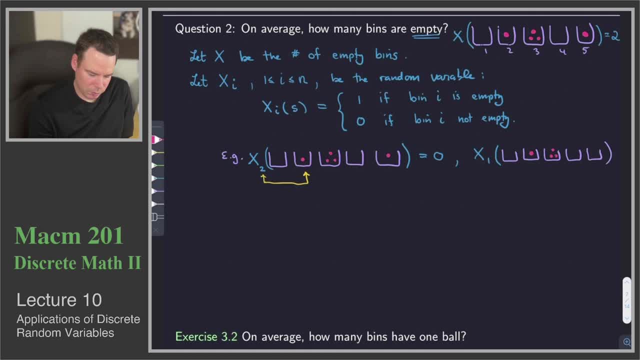 We had 1 in bin 2,, 3 in bin 3, and 1 in bin 5.. In this case, bin 1 is empty. Okay, We'll return the value of 1, because bin 1 is empty. 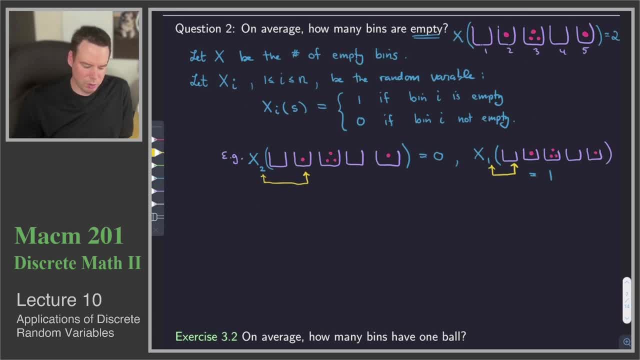 And now, if you think about this, you know it's going to return a value of 0 if the bin is not empty and a 1 if it is empty. So what we get is that the random variable we're really interested in is just the sum of these random variables. 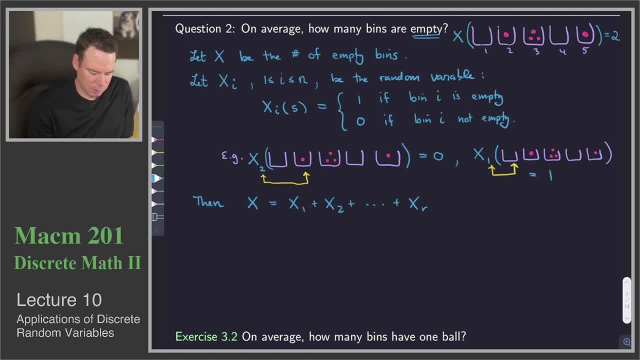 All the way up to xn, because all these random variables are going to do is just return either a 1,- yes, it's empty for that bin- Or no, it's not empty, so it will return a 0. So if I add them all up, it's just going to count the number of empty bins. 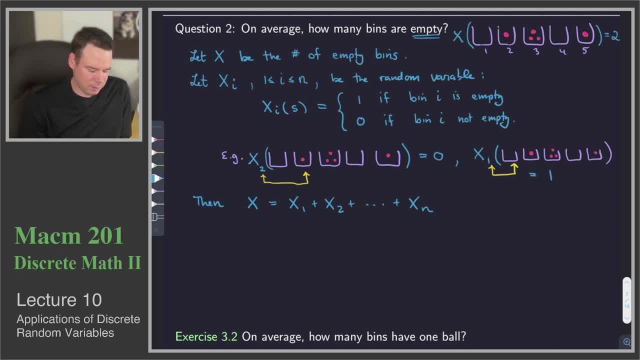 And so I've managed to write down x as a sum of simpler random variables, And so that means I can go ahead and say: what is the expected value for x? Well, by linearity, it's the expected value for x. Well, by linearity, it's the expected value for x. 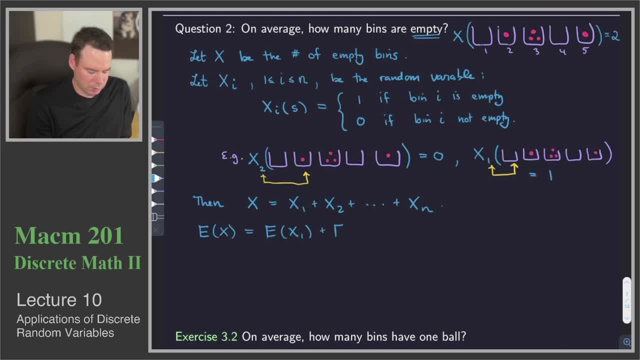 Well, by linearity, it's the expected value for x, value of x1, plus the expected value of x2, plus dot, dot, dot all the way up to the expected value of xn. and that's by linearity. So the fact that E is a linear, 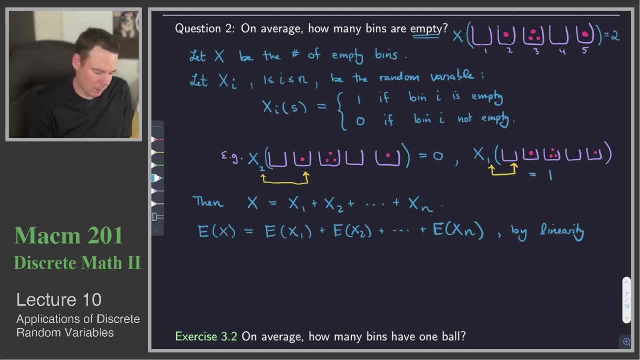 function. Now, what else can I get? Well, I get that, since E for any of the i's i only has two values in its range, either 0 or 1.. The expected value of xi is 0 times the probability that xi is 0, plus 1 times the probability that xi is. 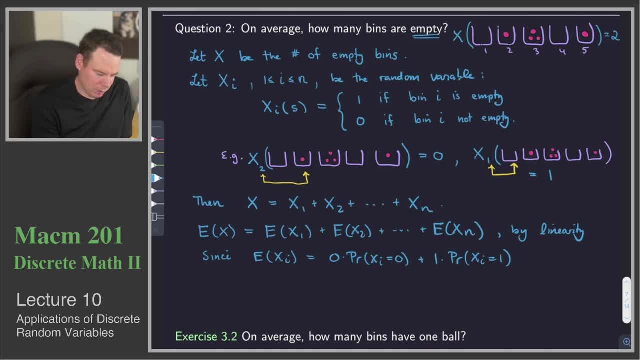 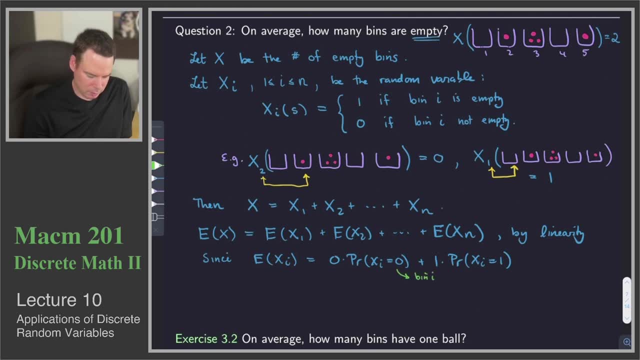 1.. But remember what these mean. xi is 0 means the bin i is not empty, Whereas xi is 1 means bin i is empty. So what is the probability that xi is 1? That's the probability that bin i is empty. 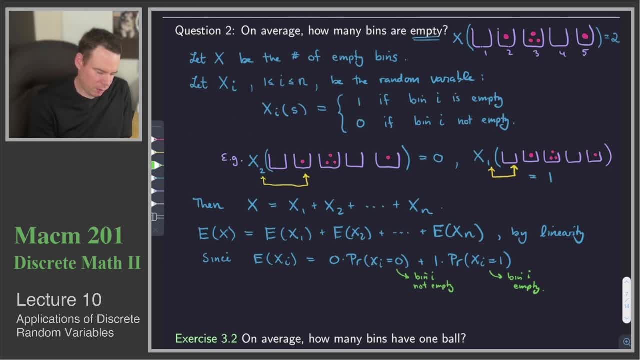 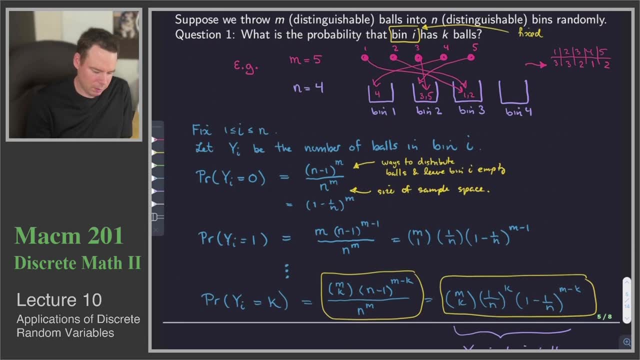 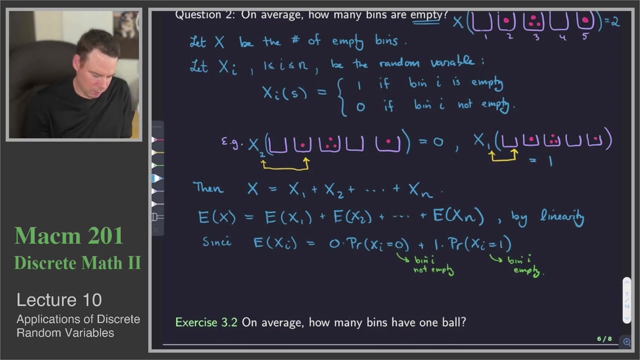 We've already worked that out. We've worked out that value above. That's this the probability that bin i has no balls in it, And so that's 1 minus 1 over n to the m. So we worked out that value already. So this is 1 minus 1 over n to 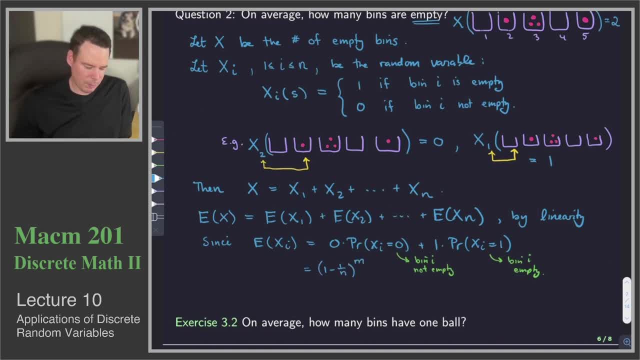 the m, and therefore we have that The expected value of x is: it's the sum of these n values, But all of them are the same. The are all 1 minus 1 over n to the m. So this is n times 1 minus 1 to the m. 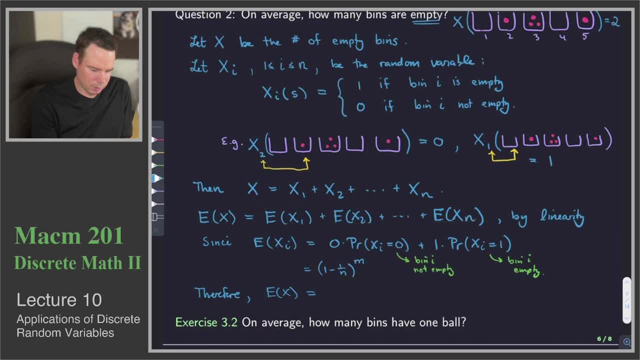 They are all one minus one over n to the m. So this is n times one minus 1 over n to the m, To the second one over n to the m. all that x is plus n value times 1 minus 1 over n to the m. 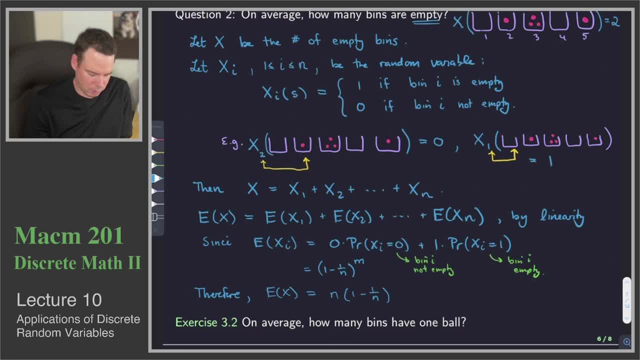 So this is n x times one minus 1 over n. up and down deals every two, two goals In Room: 1! minus 1 over n to the m. And so there we go. That is the expected number of empty bins. Now, of course, this depends on n and m. 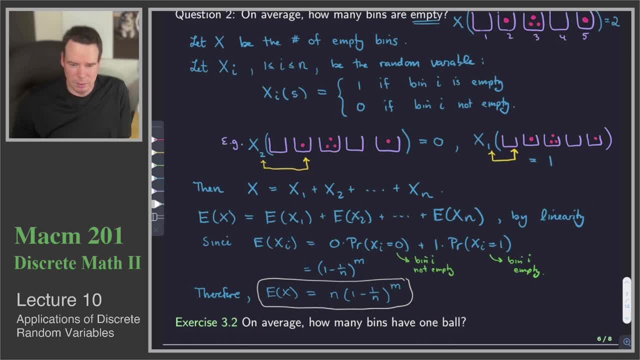 So we'd like to get a feel for what this value is. you know, how big is this, how small is this? what proportion of the bins would be empty? So I'd really like to know, you know, of the n bins. 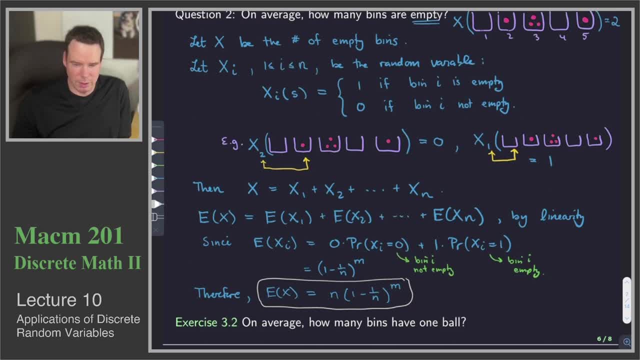 what proportion of them are empty. So this is really telling me it's 1 minus 1 over n to the m. So I kind of want to get a feel for how big this number is. That's where we can use some approximation ideas. So if I just rewrite this in the following way: 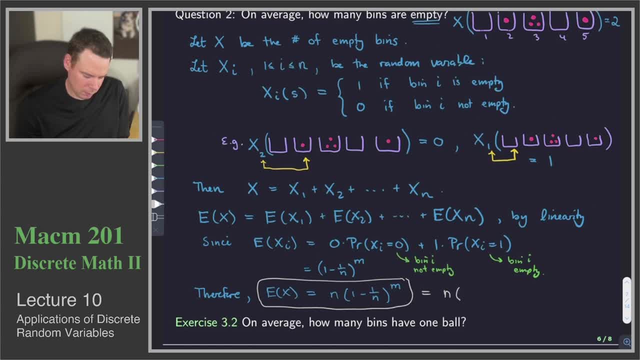 I'm going to write it as n times 1 minus 1 over n to the n, and then I will put that to the power of m over n. So all I did was insert this extra power of an n, And the reason I've done that is because now, if I draw your attention to 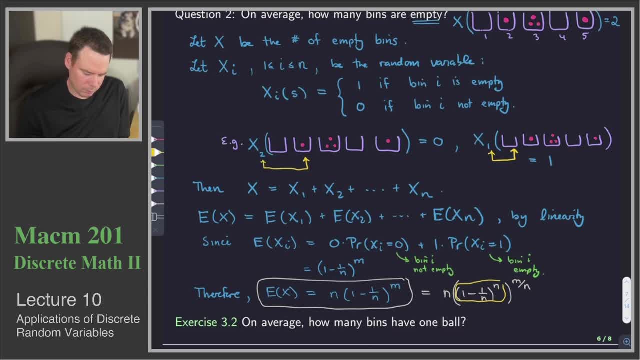 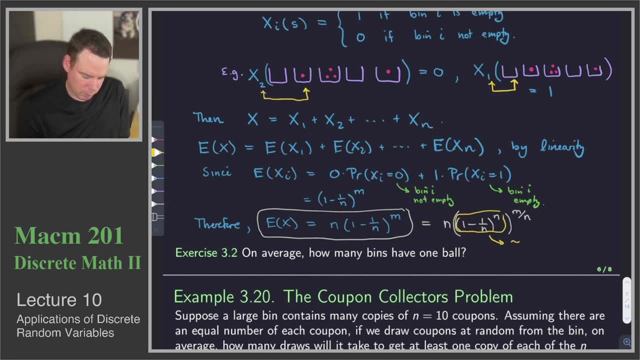 this quantity here. what we have is that this is approximately 1 over e for n large. So the limiting value as n goes to infinity of 1 minus 1 over n to the n that is 1 over e. So this is a result you would have seen in calculus. You may not remember it. 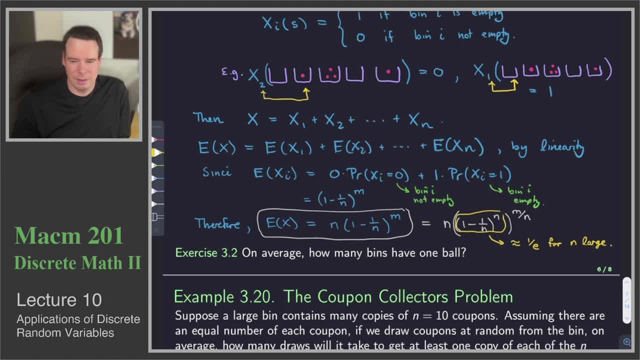 but it was certainly there in calculus. We talked about writing e as a limit one. it in fact plus 1 over n to the n, and then we could see that 1 minus 1 over n to the n actually gives us a limiting value of 1 over e. But the idea is that for n large and it doesn't have 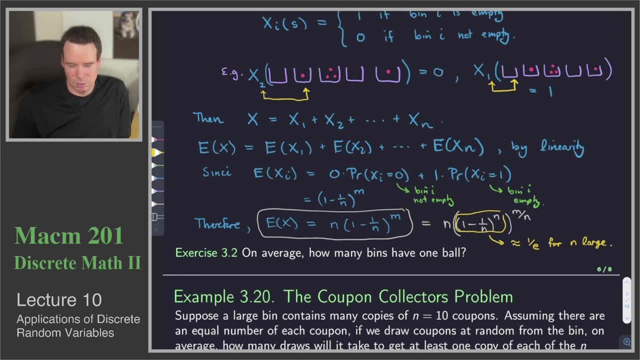 to be too large, but for n large as soon as you get it like n being 6 or 7, you're getting pretty close to e. that this is approximately e, which means that this whole thing is approximately n times e to the negative m over n. So there is a good approximation. 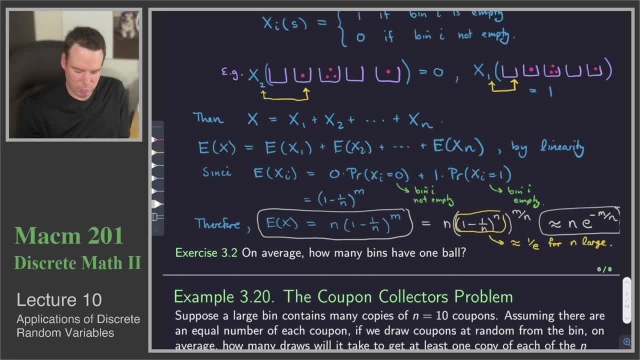 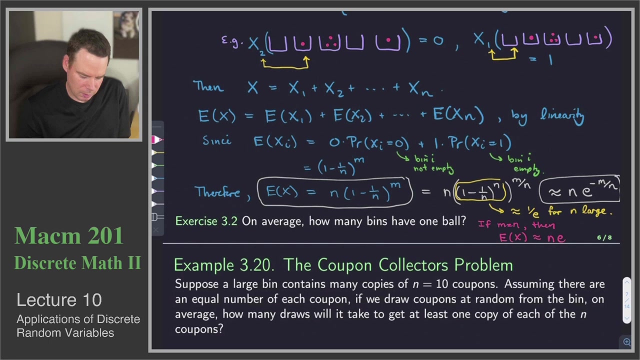 to the number of empty bins. So what that means is that in the particular case you know, if m is equal to n, you have equal number of bin to balls. then e to the x is approximately n, e to the negative 1, and that's about. 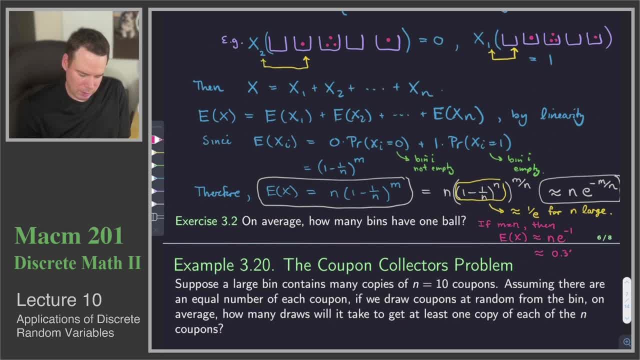 0.368, that's about. that's what. 1 over e is roughly equal to times n, So it means roughly 37 percent are empty. You know, if I had the same number bins and balls on average, I would expect to be there to be about 37 percent of them that.